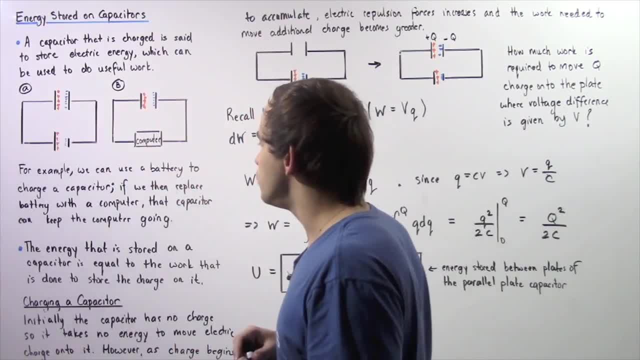 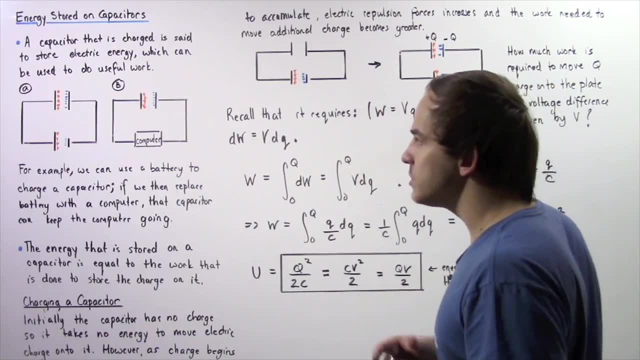 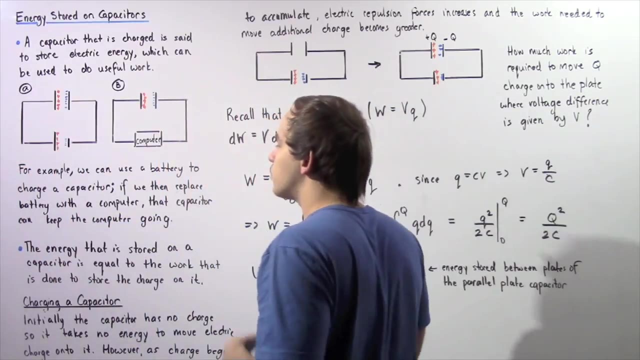 So let's see exactly how that works by looking at the following two diagrams. So diagram A essentially describes how a capacitor is charged using a battery, So a source of voltage. So let's suppose initially we don't have this battery inside our electric circuit. 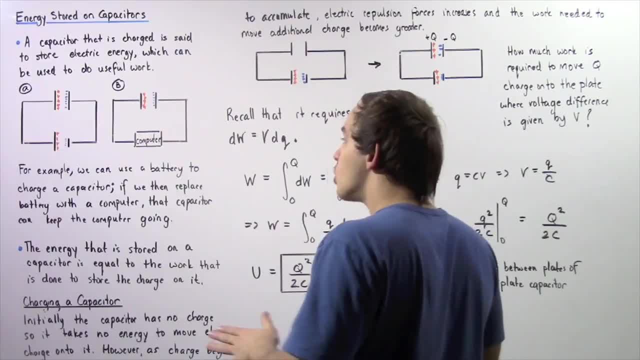 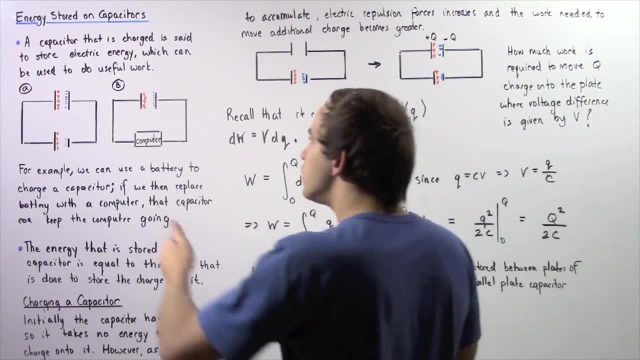 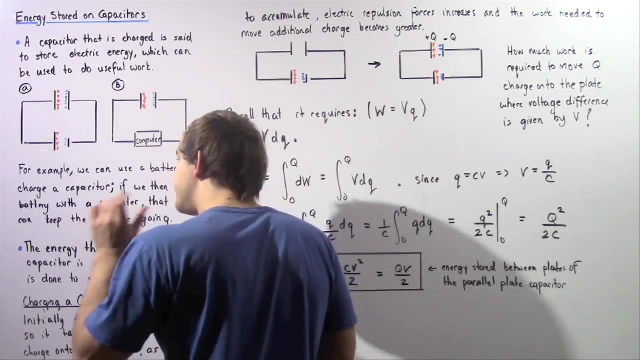 We only have our parallel plate capacitor. So without this battery the charge on either one of these plates will be neutral. So this plate will have zero charge and this plate will have zero. Now initially let's suppose we take our battery and we place that battery inside our circuit as shown in the following diagram. 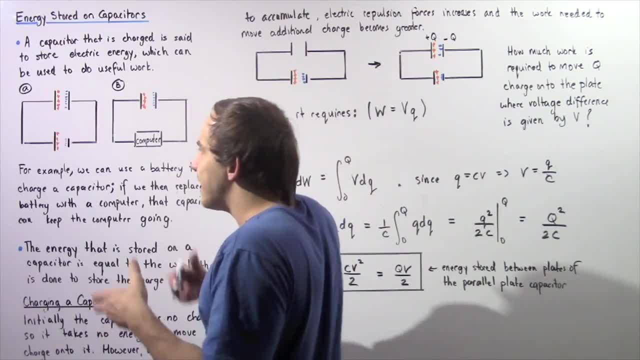 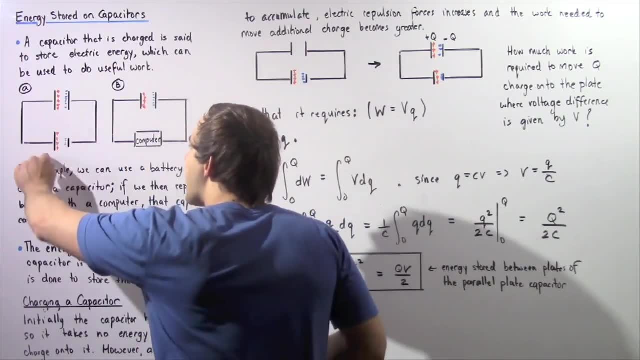 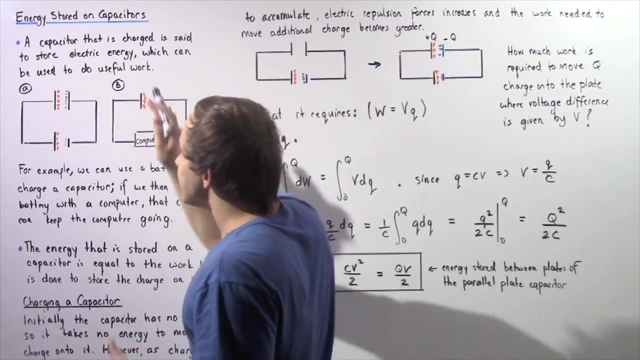 What will begin to take place? Well, essentially, electrons will begin to flow from the lower potential of our battery to the higher potential of that battery, So electrons will travel in this general direction. Now, of course, electrons cannot actually hop. 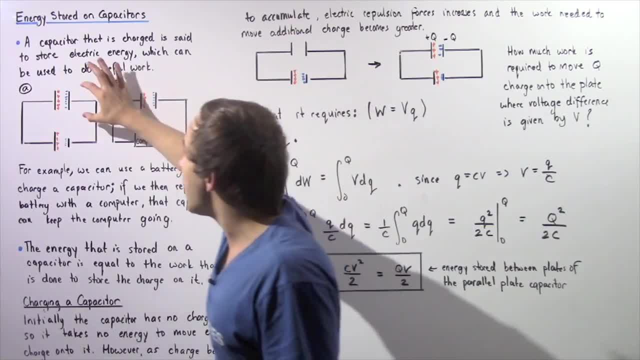 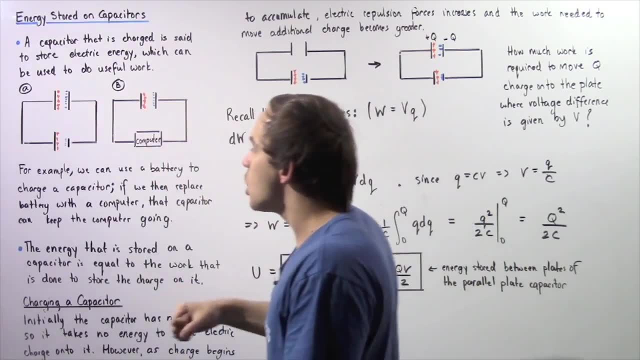 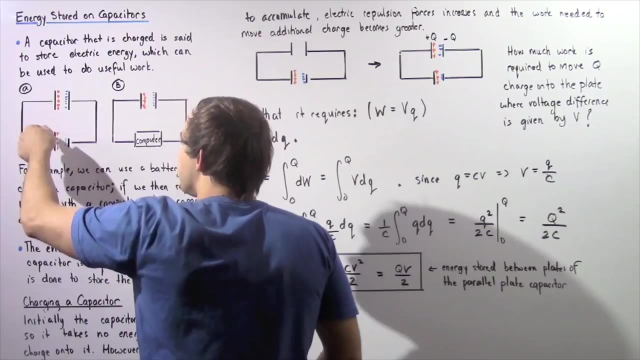 From this plate to this plate, electrons will collect on this parallel plate And the electric forces as a result of the collection of negative charge will push the electrons on this plate away And those electrons will now travel to this plate and will accumulate on this plate of our battery. 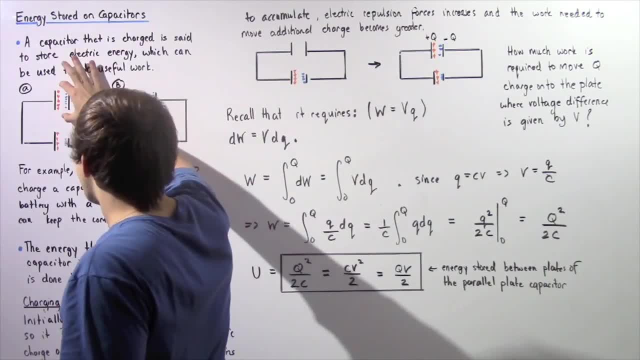 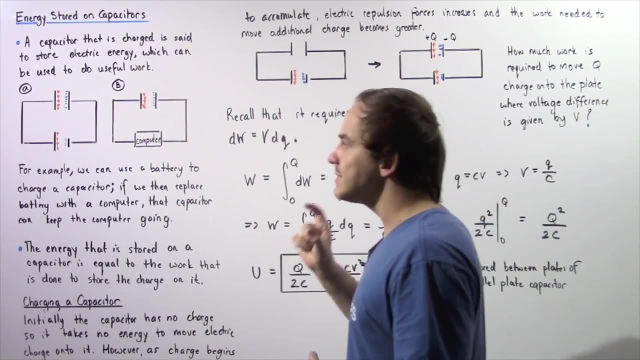 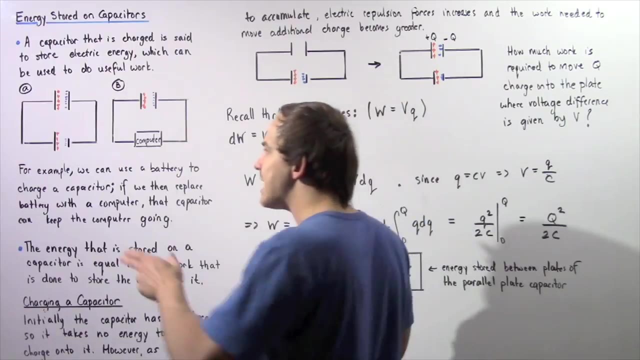 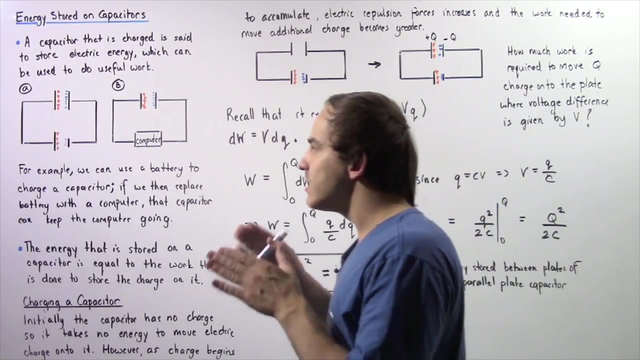 Now, eventually, the voltage that is reached by our capacitor will be the same as the voltage of the battery, And at this point our capacitor is said to be fully charged. So now our capacitor is fully charged, And let's suppose we take our battery out of our circuit and instead we place into our circuit a certain device that requires electricity. 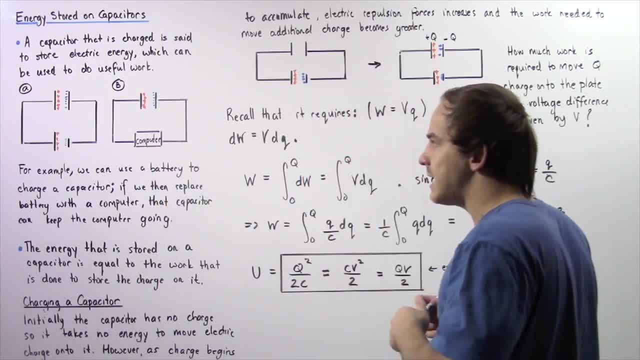 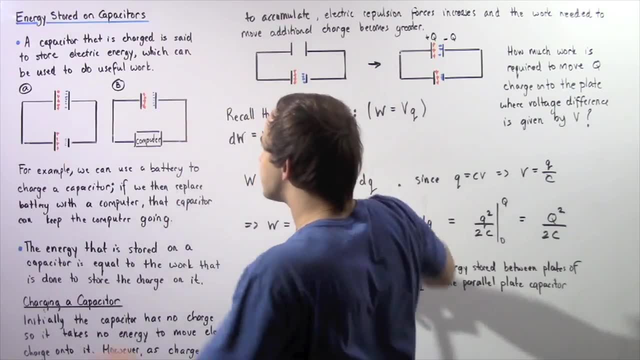 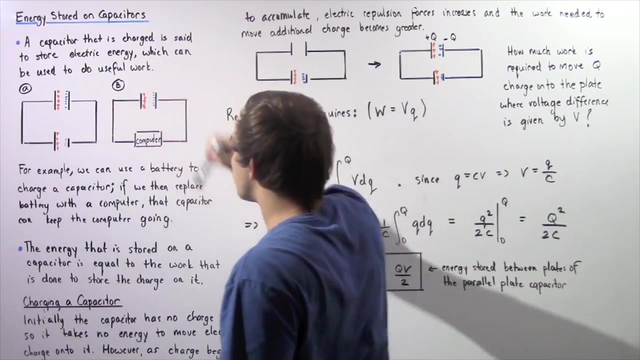 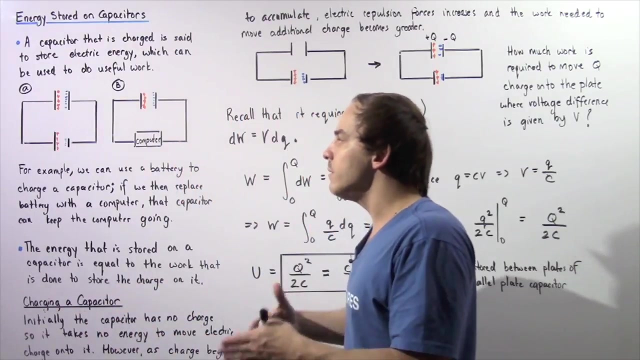 For example, a computer. So what will begin to take place is electrons will begin to flow from this lower potential plate of our capacitor To this higher potential plate of our capacitor. Electrons will begin to travel in this direction And because electrons will begin to move, the movement of those electrons will be able to do useful work on this computer. 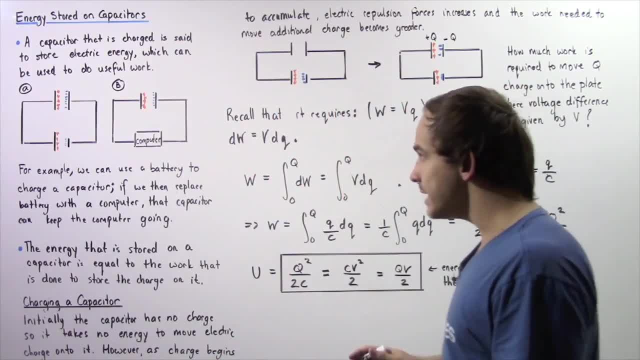 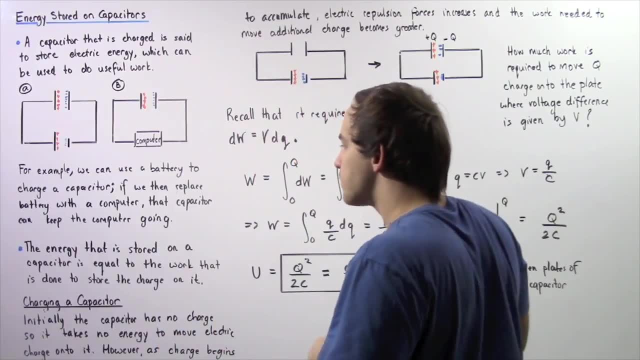 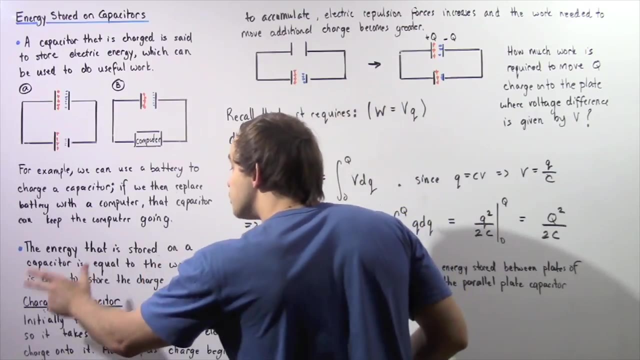 And that will, in turn, power our computer. Now, what exactly is the energy that is stored in our parallel plate capacitor? Well, the energy, The energy that is stored on our capacitor, is equal to the work that is done to bring all that charge from this plate onto our capacitor. 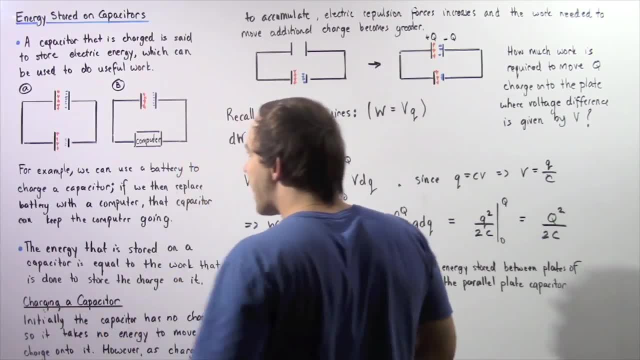 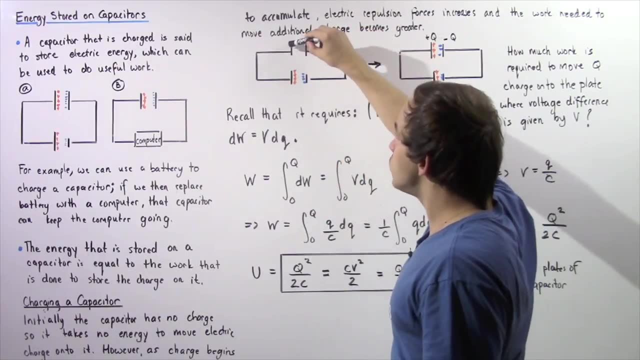 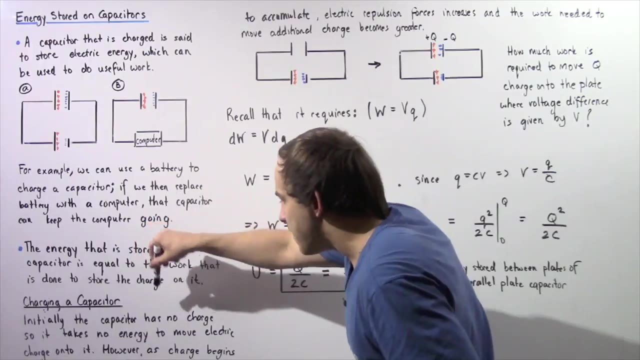 So let's examine once more how charging a capacitor actually takes place. So what takes place initially? So initially, we know that these two plates of our capacitor have absolutely no charge. So that means initially. So that means initially. 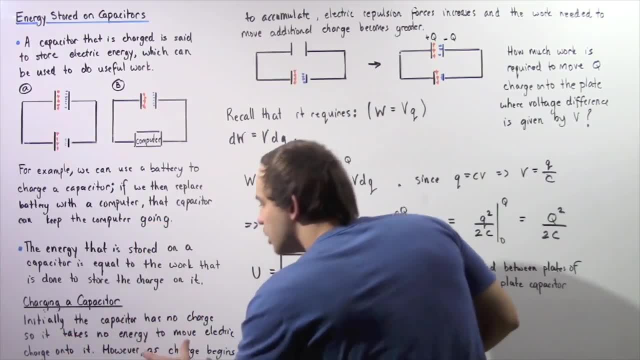 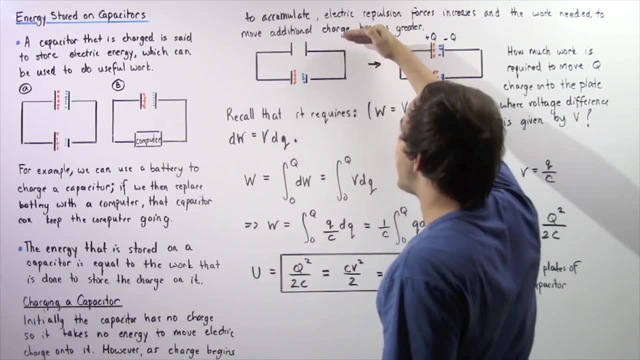 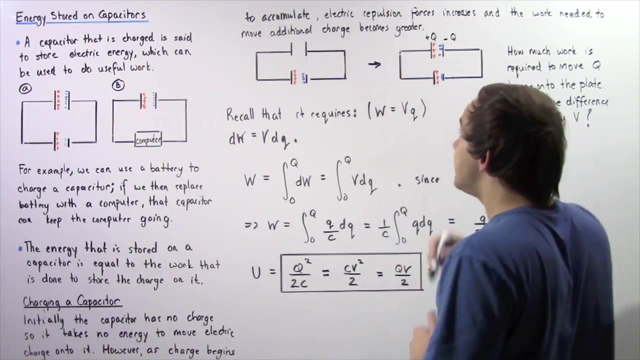 the capacitor has no charge, So it takes no energy to move electric charge onto those plates. So initially these electrons flow without any energy onto our plate Without any energy input. However, as the charge begins to accumulate on this plate, more and more electrons appear on this plate. 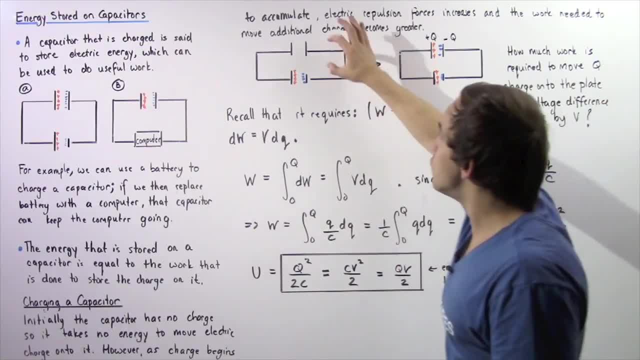 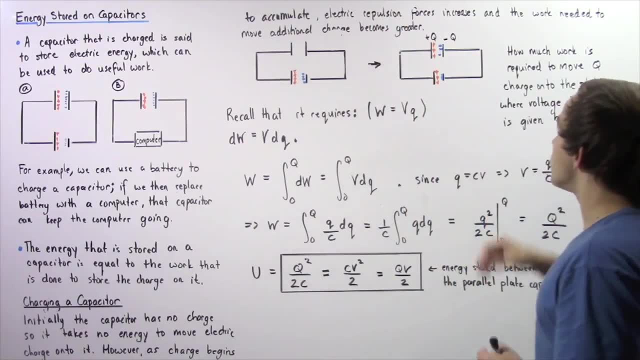 So electrons find it more difficult to move onto a region where there is a larger negative charge. So electric repulsion forces increase and the work needed to move those additional electrons becomes greater. So of course eventually this will be fully charged where this plate will have a negative Q charge and this plate will have a positive Q charge. 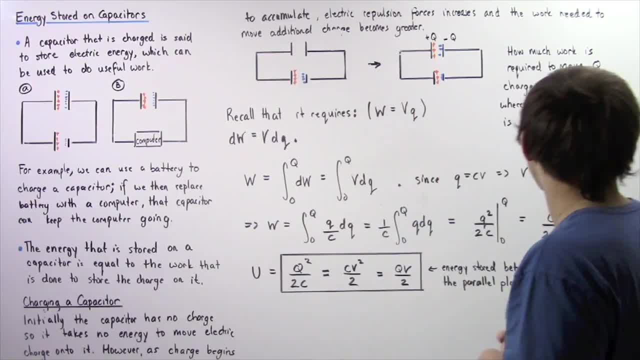 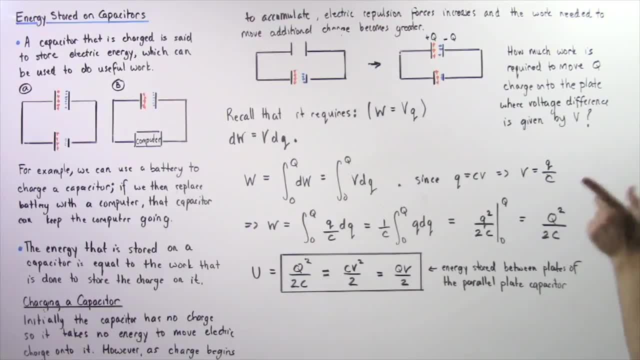 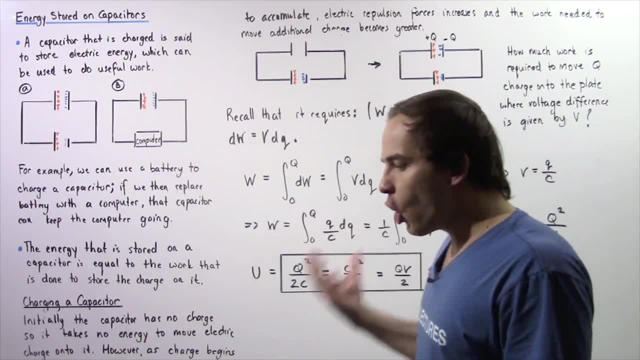 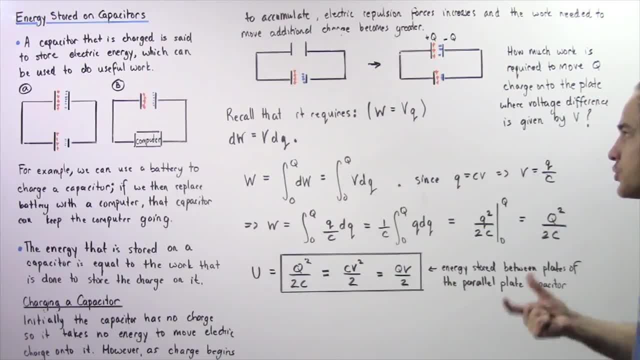 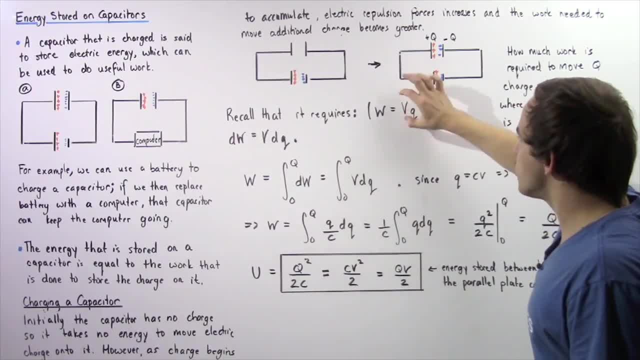 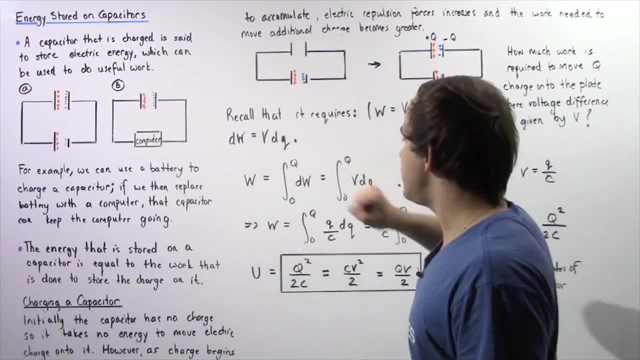 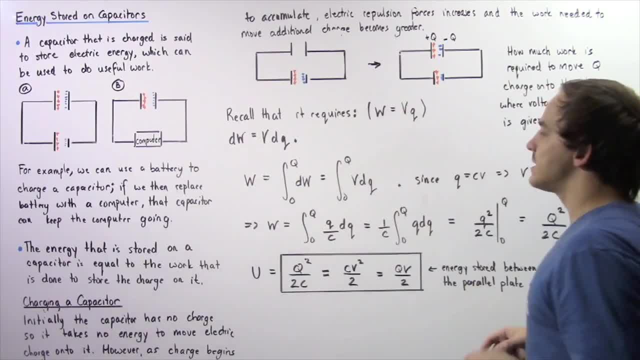 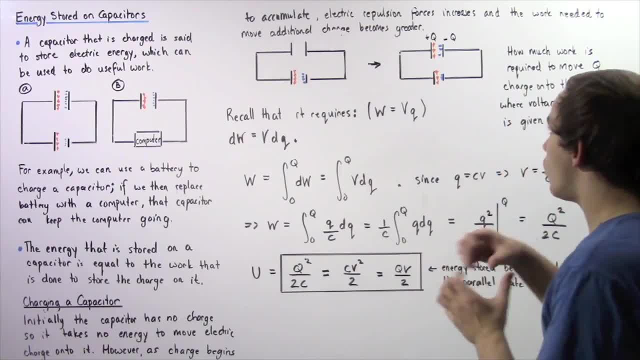 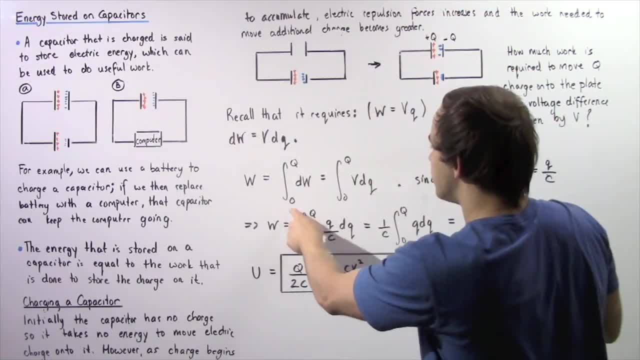 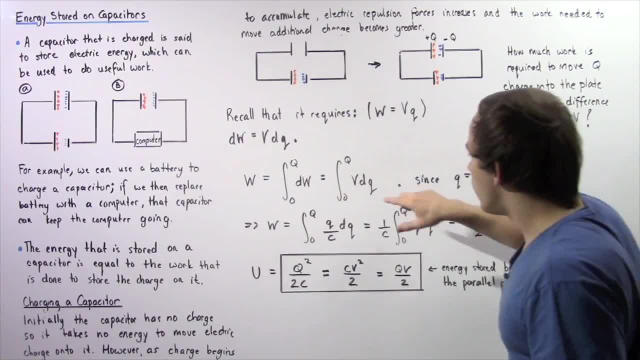 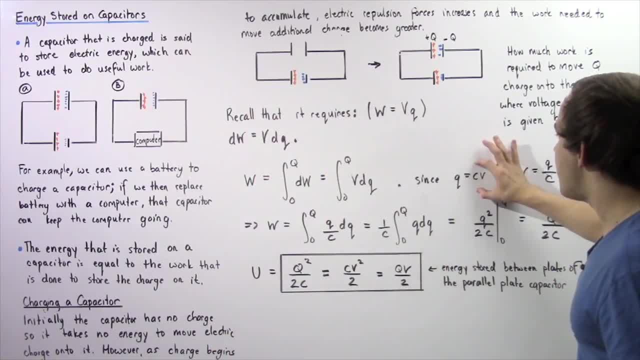 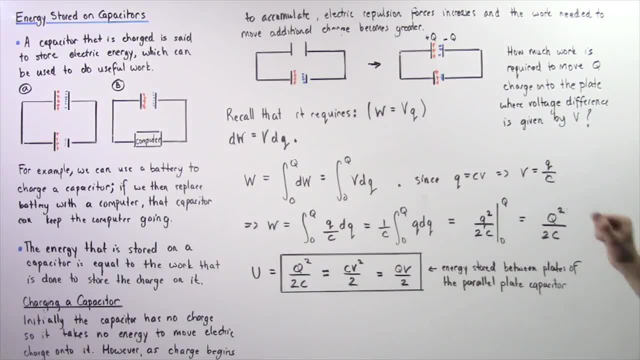 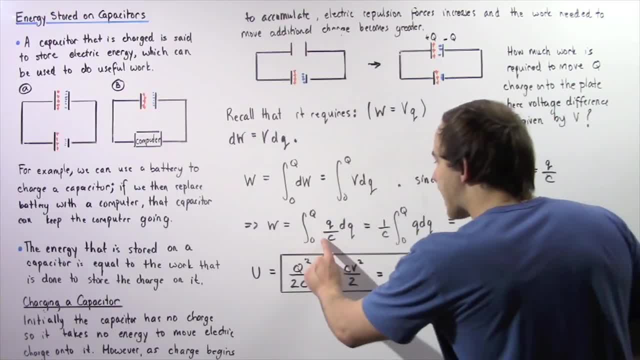 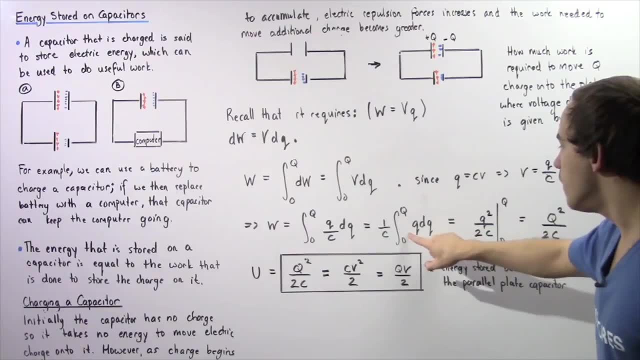